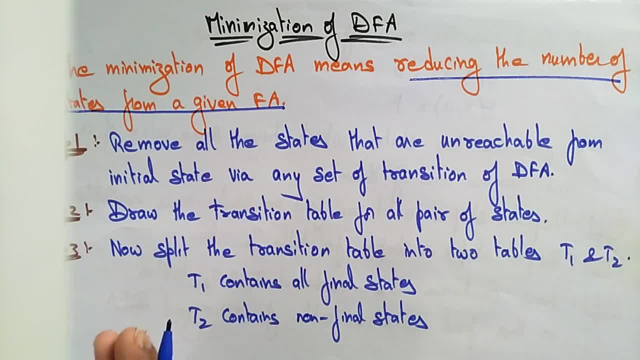 Okay, so now let's see the steps that has to follow for minimizing the DFA. So in this video I just give the algorithm. that is, the basic steps that you need to follow for minimization, and the next video I will explain with an example. Okay, so let's try to explain. 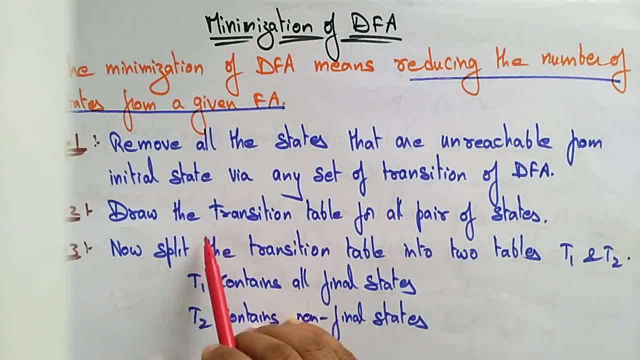 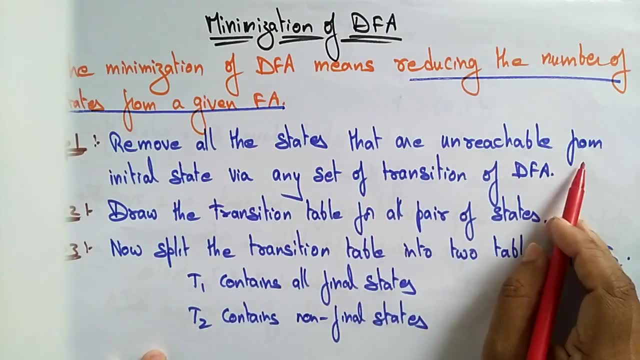 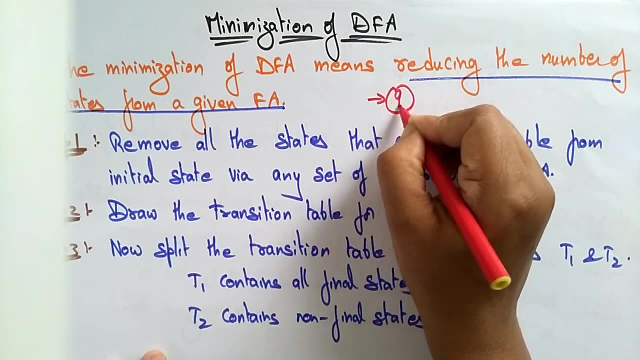 let me try to explain the algorithm: minimization of deterministic finite automata. the first step: what you had to do: remove all the states that are unreachable from initial state via in any set of transition. what it mean, suppose if, if q1 is the initial state, okay, some q1. it has to reach all the 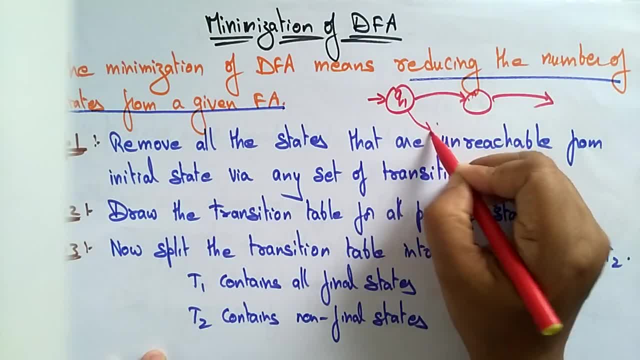 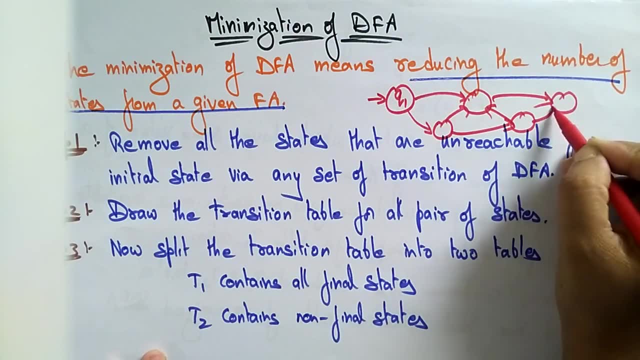 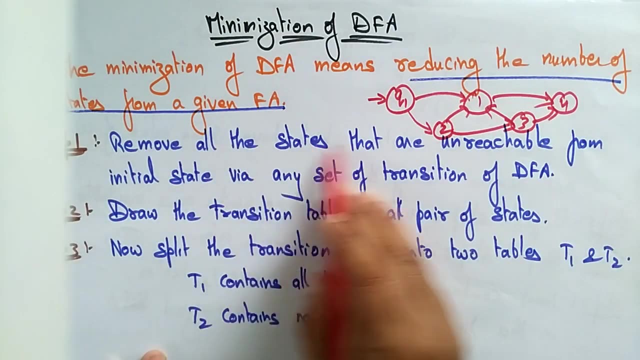 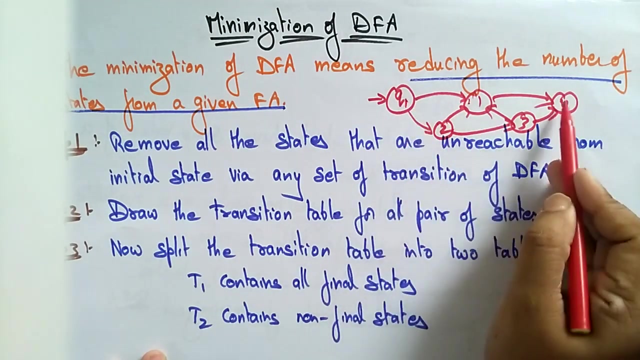 states, it has to reach all the states that are participating in the network. okay, so like this, let me do. okay. so here one, two, three, four different states are there. so here, first is remove all the states that are unreachable. so here, from q1, one is reaching. okay, if you one wants to reach 4, it can reach via any set of. 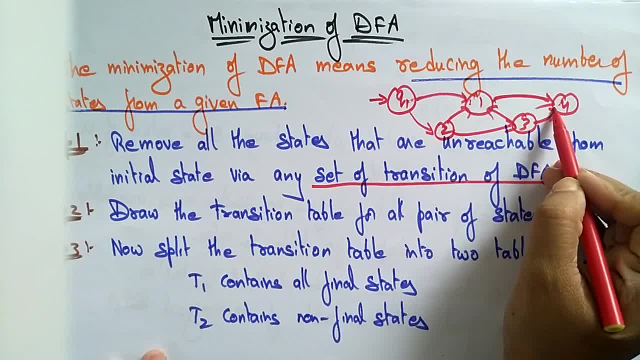 transitions. so from 1 to 4, it is going to reach. okay, if you want to reach 2, it can reach. if it want to reach, it can reach. it want to reach 4, it can reach. suppose here this direction is like this: okay, so this is the 4 and it is coming. so here, remove all the states that are unreachable. so 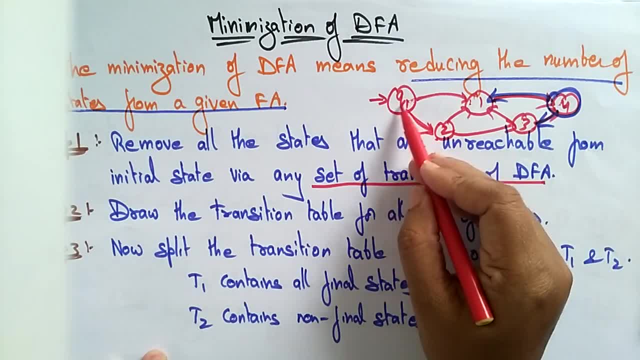 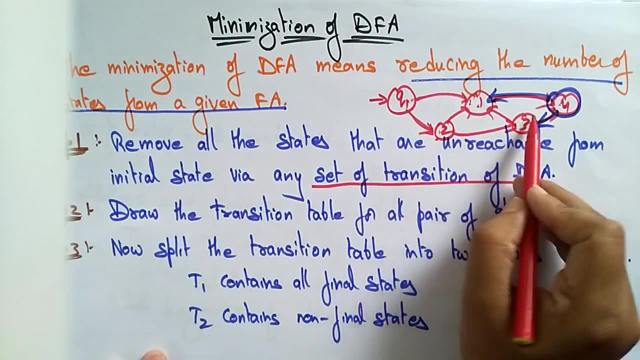 from q1 to. i want to go to 4, so can i go this way? it is not possible. now let's check here: from 2 to 3, okay, 3 to 1 i can go, but 3 to 4 i can't go because 4 is coming to 3 side. so here the 4 is. 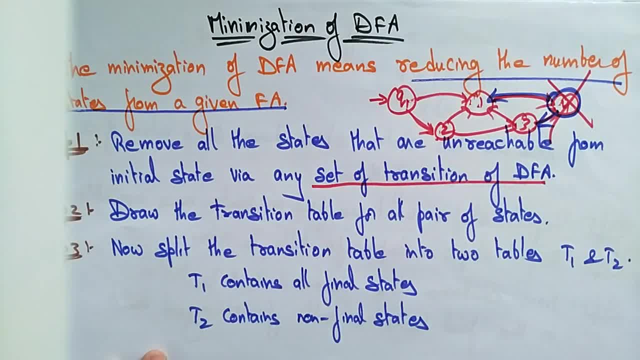 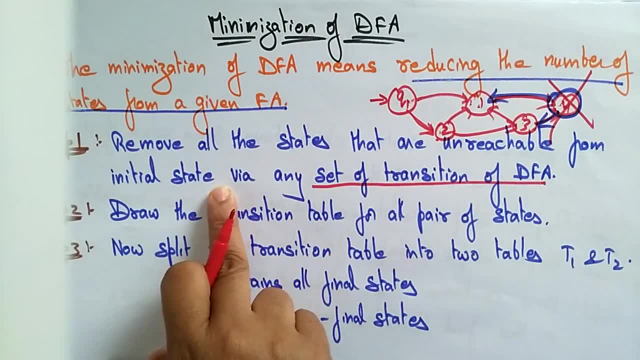 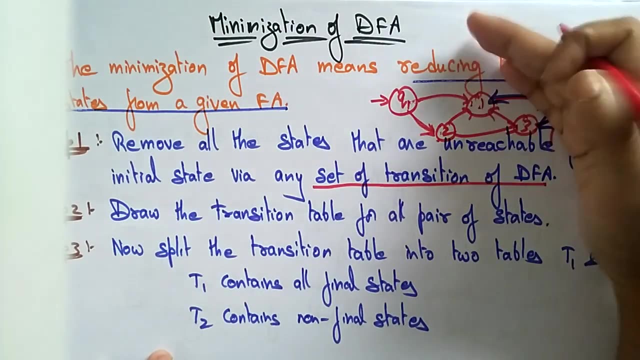 unreachable. so just remove that 4 from the transition. so that is the first step. remove all the states that are unreachable from initial state, from initial state to which state is not unable to reach. just remove that transition from the, that node from the transition. that's first. 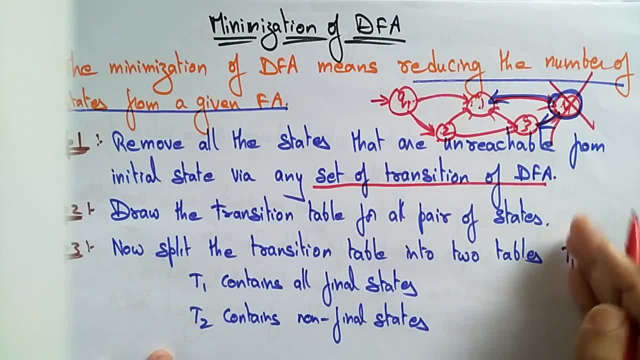 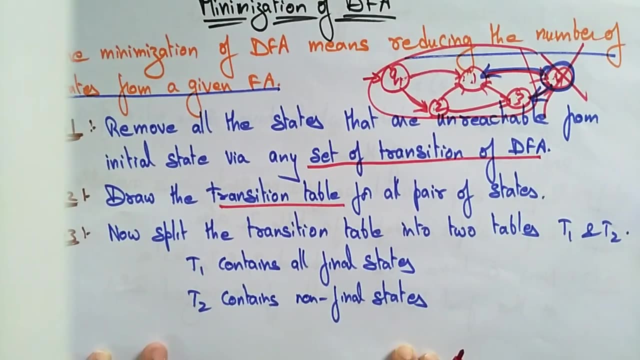 second, draw the transition table for all pairs of states. so, after removing this state, draw the transition table for the remaining states, the remaining states, whatever, that are participating in the network. those states has to further. you need to draw the transition table. okay, next, now split the transition table into. 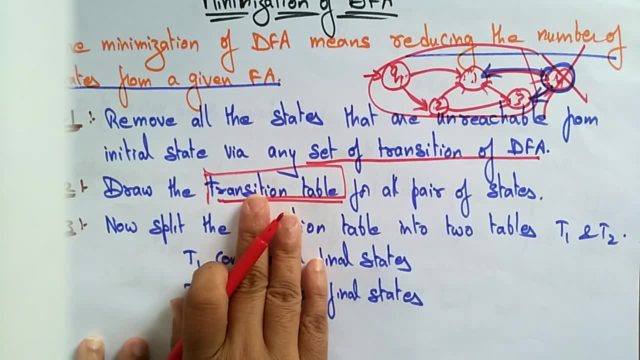 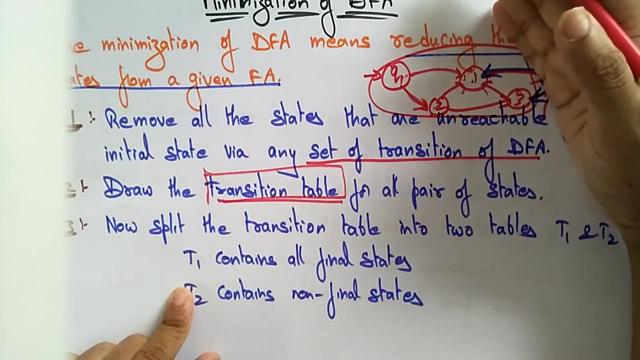 two tables. so whatever the transition table, i got that table. i want to split into t1 and t2 why i am splitting. okay, let me tell you first follow the algorithm, then you can. after seeing the example, you can clearly understand. so, after removing the unreachable state, 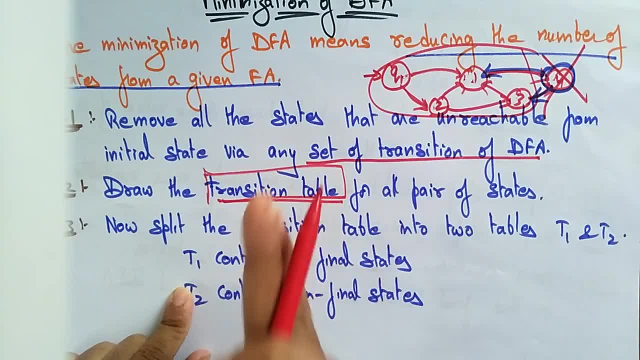 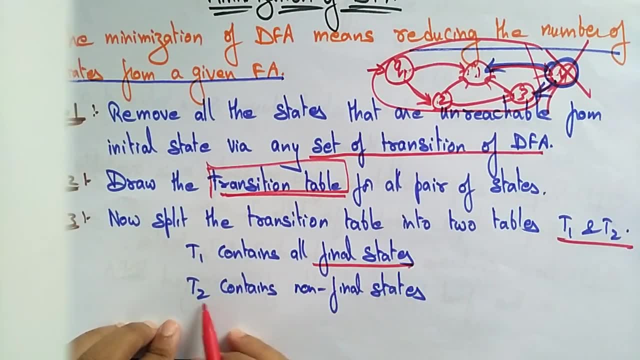 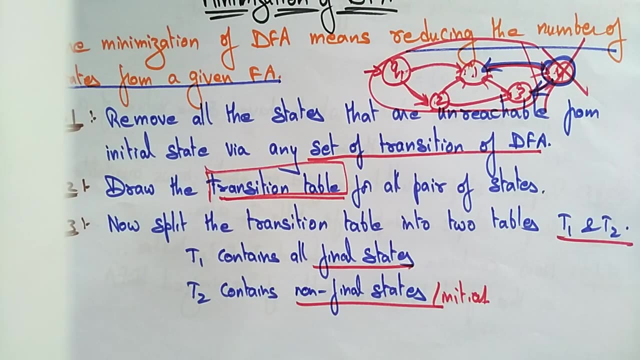 i draw the transition table. so i am splitting the transition table into two tables, t1 and the t2. now t1 contains all final states and t2 contains non-final state means. here the initial state is also there, non-final state and initial state. so t1 suppose in a deterministic finite automata. you. 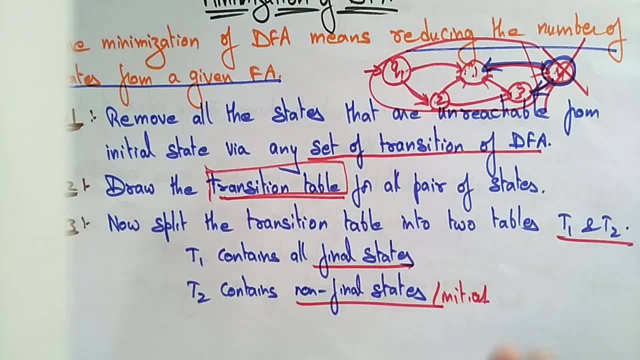 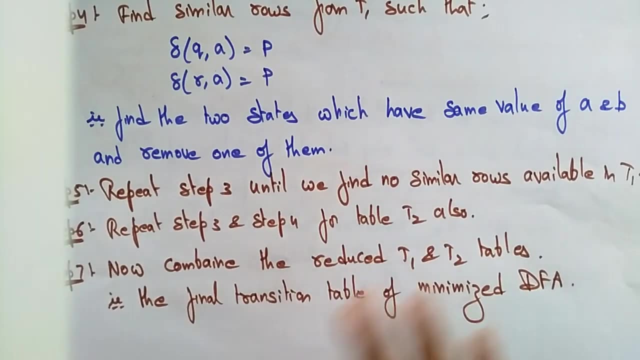 know that. so if all some, whatever the final states that are there, that final state should be is one table and the remaining initial and intermediate state will be in another table: t1- t2. t1 contains all final states. t2 contains non-final states. now step 4. okay, i divided the two tables. one 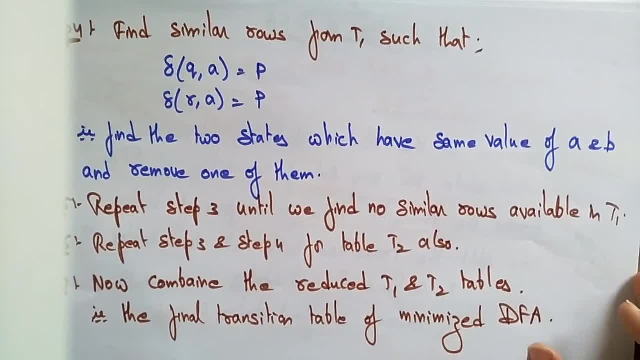 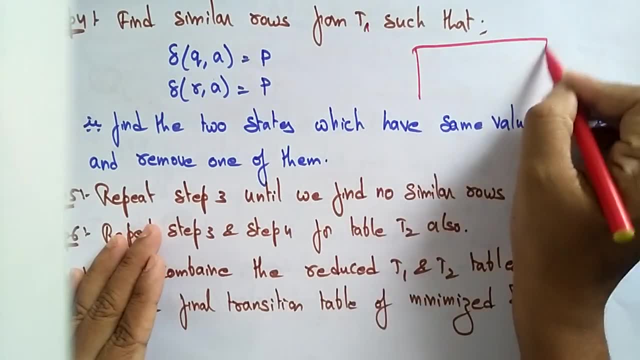 transition table into two tables. next, what i have to do now: find similar rows from table t1. so if you take the t1 you need to find the similar rows. i have drawn the transition table right, so in this i need to find the similar rows. so that is. 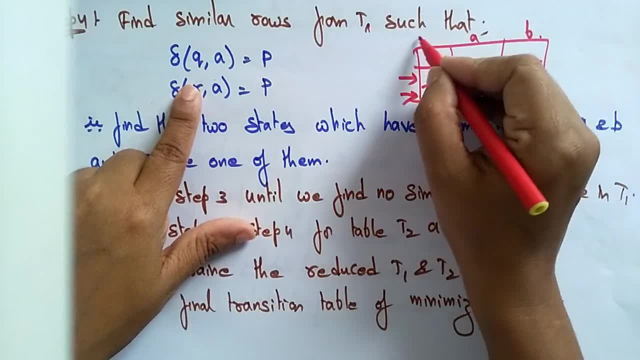 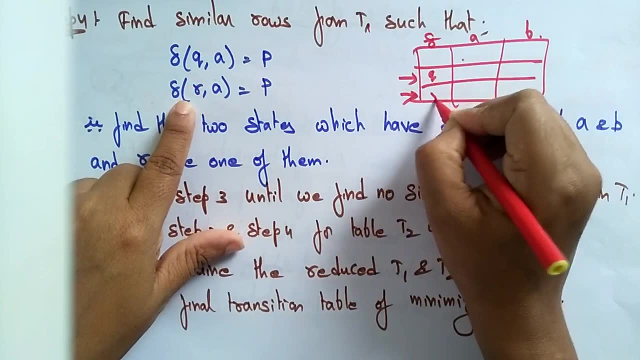 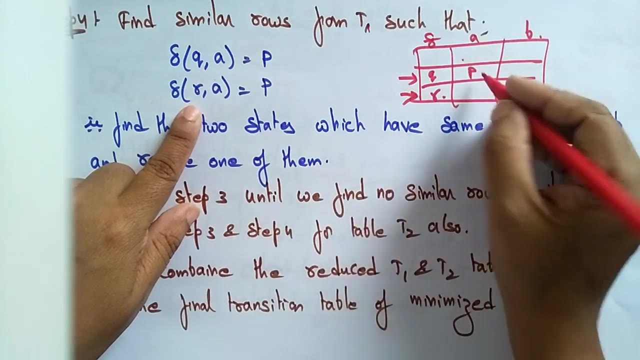 the transition function. let's say a and b is the input and this is the transition function you get. okay, you will get here the transition function. if transition function- let me take q and r- if transition function of q, a is equal to the p and the transition function of q on a is equal to p, 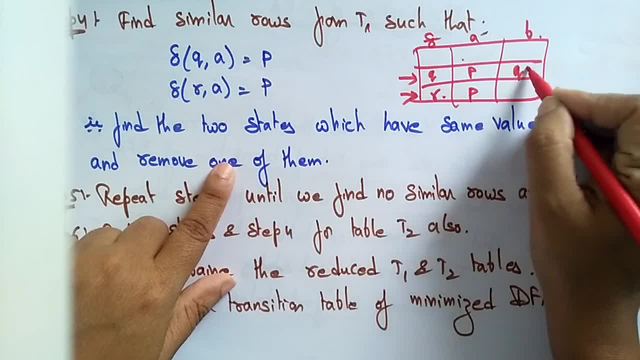 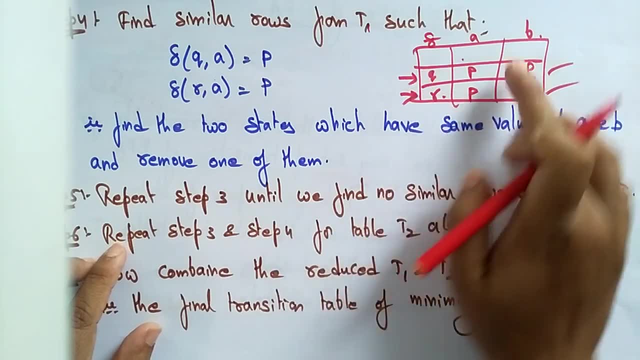 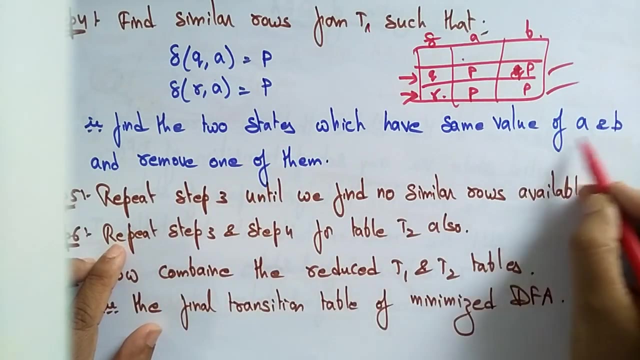 so here also you will get the same uh, p and p. okay, if you are having the similar rows. so this q and r is having the similar rows, p, p, p, p. okay in this case, that is, find two states which have the similar values of a and b. a and b is having. 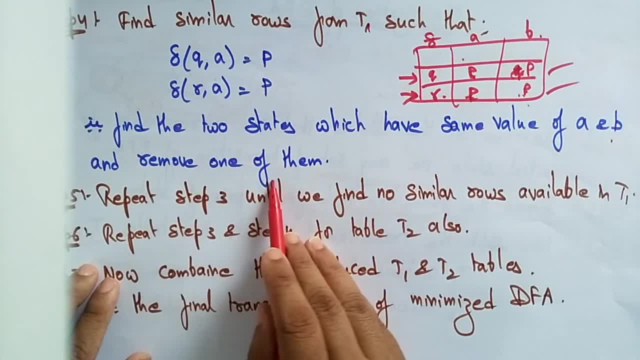 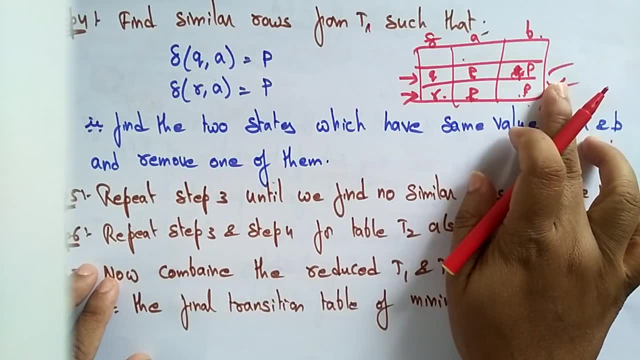 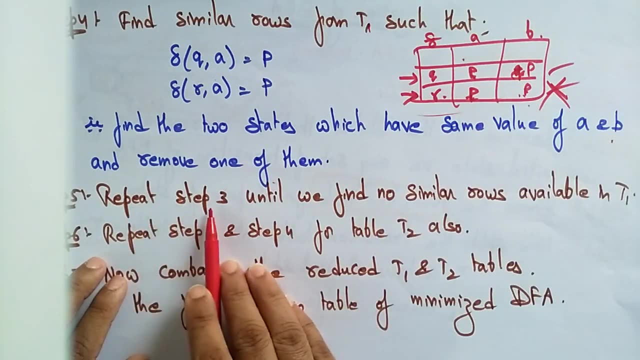 the same, similar value, same states, p, p, p and remove one of them. so here these two are equal, so just remove one. one state, one row. you have to remove means i am reducing, i am minimizing my table, so remove one and replace here. repeat step three until we find no similar rows available in.